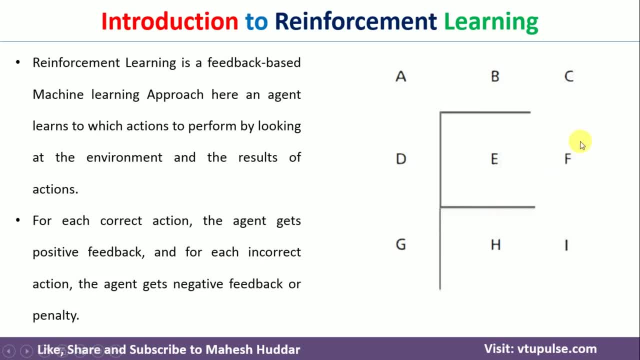 it is a correct action. he will be given some positive reward here. Now, when he comes to this particular thing, he will look into this particular environment and then he will perform one of the action. The one action is: either he can perform up or he can perform down here. 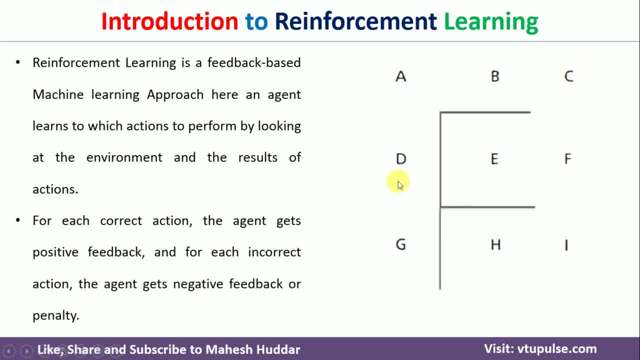 Whenever he performs up, the meaning is, again, he is going towards this particular G and G. the meaning is it's a correct action. For this one also, he will be given a positive reward or a positive feedback here, But when he performed this action, that is from F to. 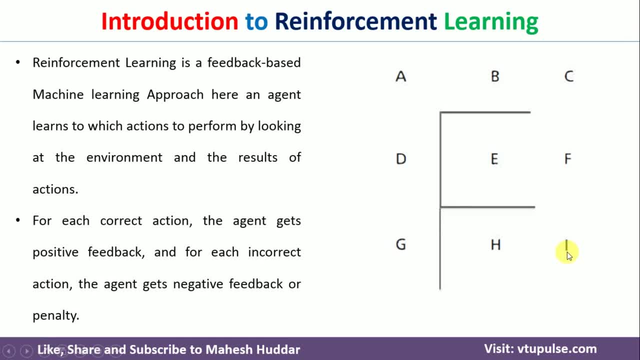 I. the meaning is: this is incorrect action. For this one, he will be given a negative feedback. So whenever a negative feedback is given, he will understand that he should not follow such path in future. over here, So that is how reinforcement learning works. 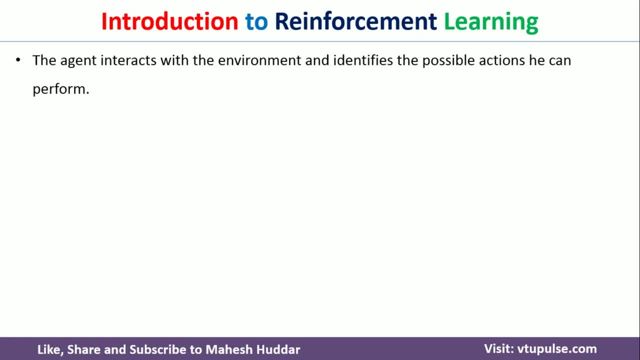 in this case In reinforcement learning. As I said earlier, the agent will interact with this particular environment and then he will identify one of the possible action And then he will perform that particular action over here. For each of those particular action he will be given a positive or negative feedback. 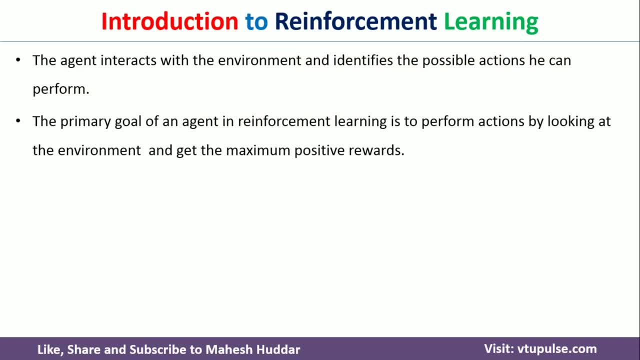 in terms of rewards, The main goal in this case is to get the maximum rewards as as much as possible. over here In reinforcement learning, we don't have any label data. That's the reason he has to learn through his experience. for example, if he is getting a positive reward, the meaning 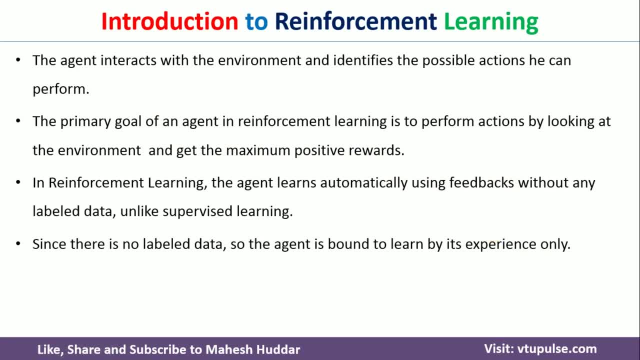 is it's a correct action. If he is getting a negative reward, the meaning is it's incorrect action. So through this experience only the agent will learn. in this case, because we don't have anything called as a label data over here, But in supervised machine learning. 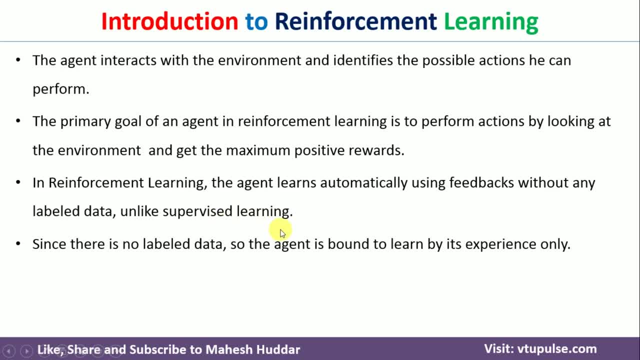 technique. we have a label data. using that label data, the algorithm will be trained over there. So in that case the experience doesn't matter much over there. Reinforcement: reinforcement learning can be used to solve a specific type of problems where the decision 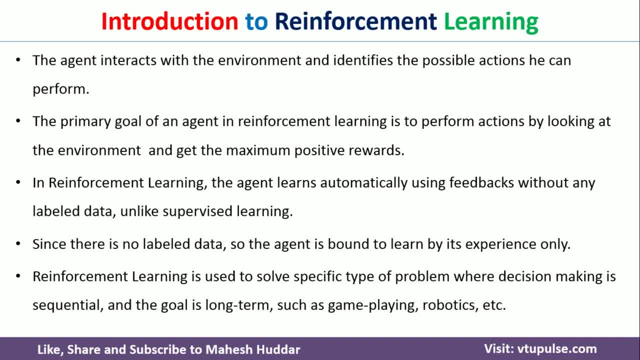 making is sequential, that is, step by step. if you look at that previous example, the agent will reach that particular goal step by step. in that case, he cannot go directly to that particular goal in that case. so that's the reason: if the decision making is sequential, we can use reinforcement learning as well, as it should be a long term, like you cannot. 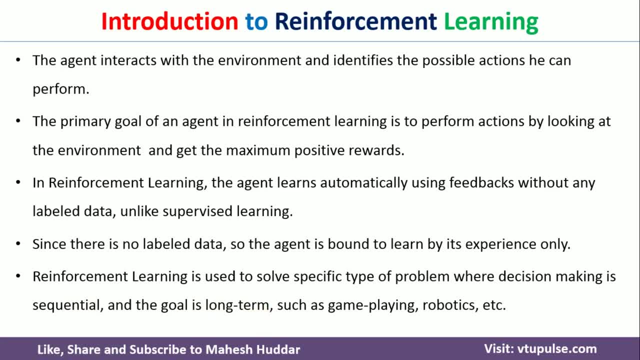 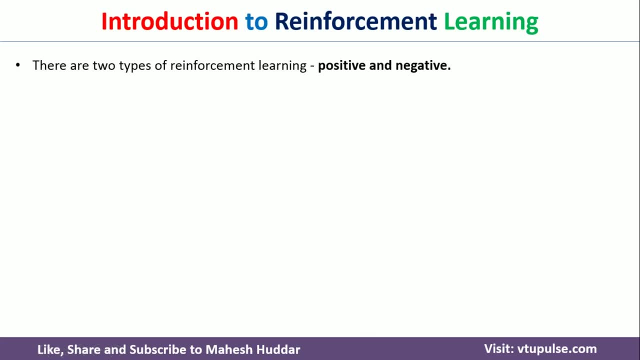 expect the result immediately in this particular case. so if it is a long term goal, then you can use the reinforcement learning in that case. some of the examples where we can use reinforcement learning is game playing, or we can use it in robotics also. there are two types of reinforcement learning. we have one is called as positive reinforcement learning. 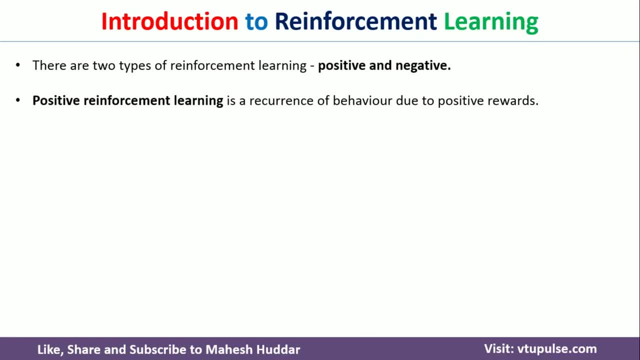 and second one is called as negative reinforcement learning. positive reinforcement learning is a recurrence of behavior due to positive rewards. in this case, recurrence means the same behavior will be repeated again and again. the reason here is we have got the positive rewards, in this case the positive rewards. 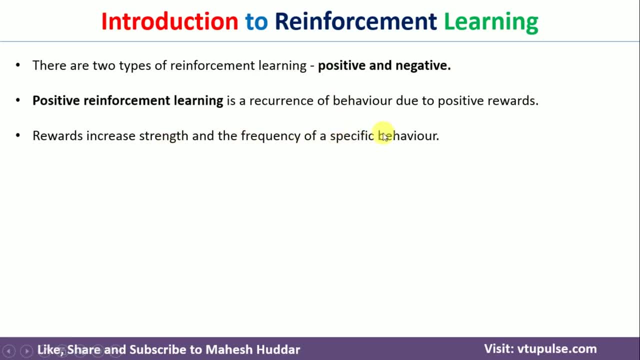 increases the strength and the frequency of such actions will be repeated in the future over here because we got the positive rewards in this case. that is what has been written here. these positive rewards encourages the agent to perform the same actions and get the maximum reward over here. similarly, the negative reinforcement: learning- is the deterrent. 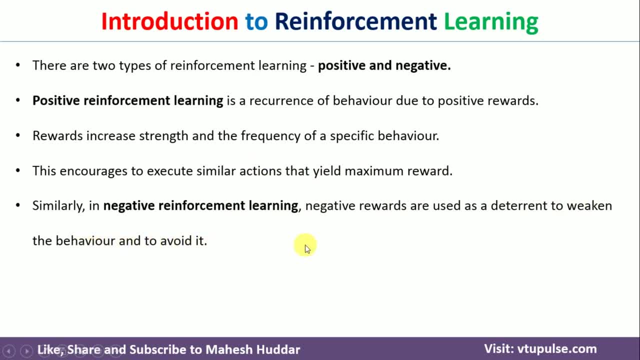 to weaken the behavior and to avoid that particular action to be performed in the future over here. that is, whenever you have given a negative reward, it will deterrent the action what has been performed over here and then it should, but not be performed in the future over here. 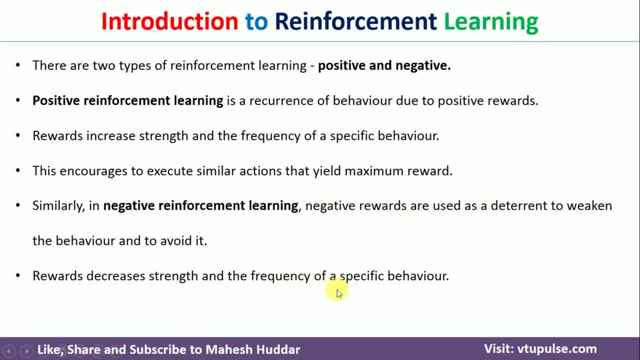 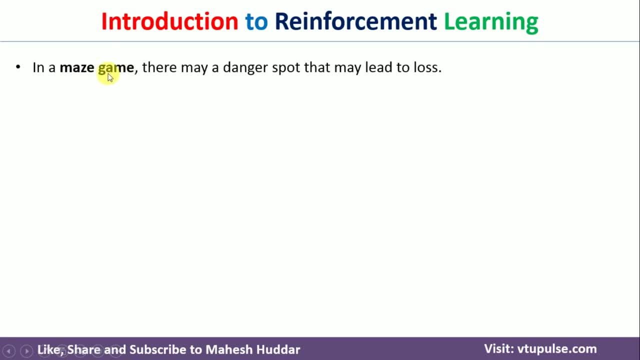 this. negative rewards will decrease the strength and such action should not be performed in the future. let us take an example of a mage game. in this particular mage game, let us assume that there are some dangerous spots are there. whenever the agent has gone to dangerous spot, the meaning is he will lose. 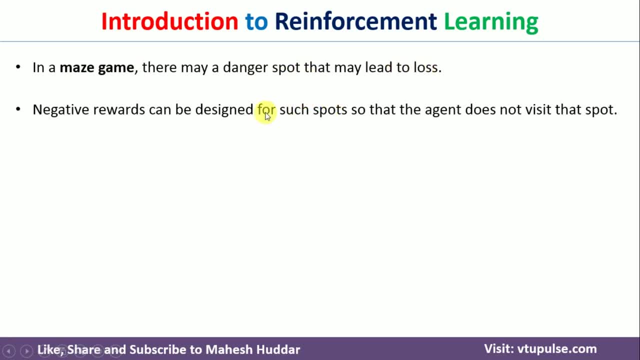 that particular game. so the thing over here is the agent has to avoid going to that particular dangerous spots because whenever he go to that dangerous spots he will be given a negative rewards. in this case, let us assume that whenever he goes to that particular dangerous spots, so he will be given a minus 10 points and if you perform a correct actions, let us say 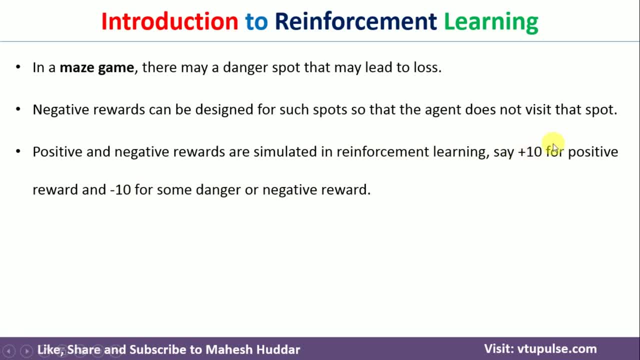 that he will be given a positive 10 points. so positive 10 points will be given to. the 10 points will encourage the agent to perform such actions and a negative 10 point will discourage the agent to perform the actions, which will lead to what you can say that the danger spot or the 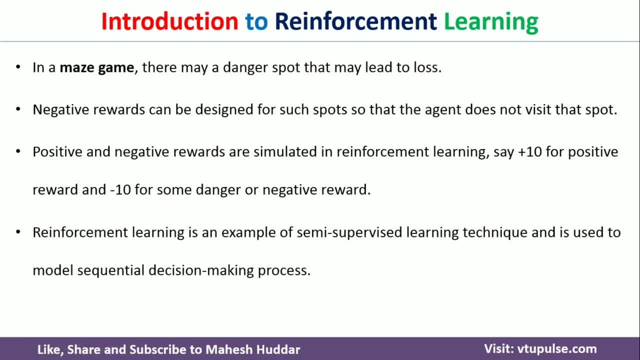 person may lose the game over here. the reinforcement learning is an example of semi-supervised learning. you cannot say that it is a supervised machine learning technique or it is unsupervised machine learning technique, because in supervised machine learning technique we have a label data. in unsupervised machine learning technique we don't have any labels over there. but in reinforcement 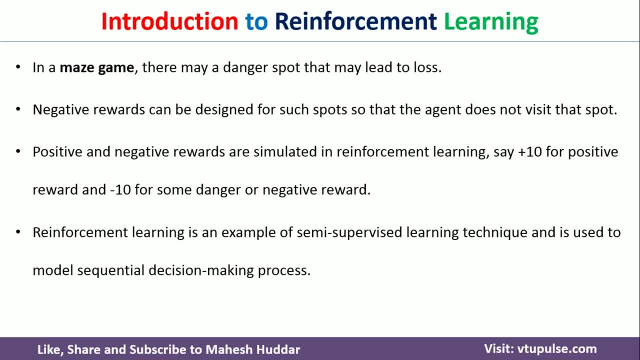 learning we have. we don't have complete label data and we we cannot say that there is no one to supervise here. definitely the environment is there and then these rewards will encourage or discourage to perform some actions. so that's the reason we can say that the reinforcement learning 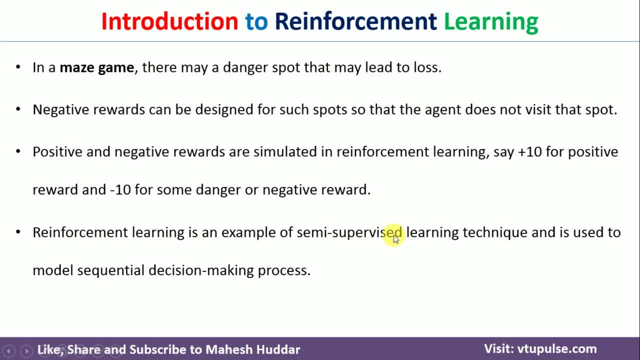 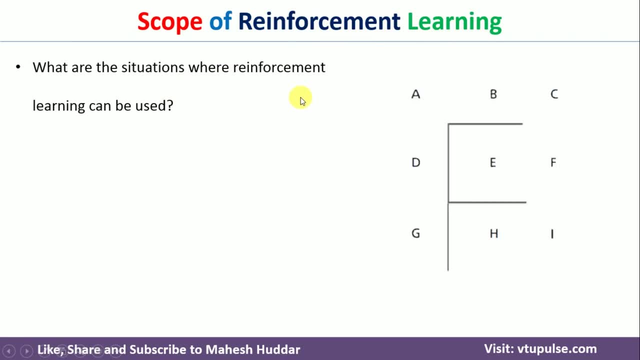 is a semi-supervised machine learning technique in this case. now the question is where we can use this reinforcement learning. we can use this reinforcement learning technique to solve games, or if you are designing a robot. in such cases, we can use this reinforcement learning. let us take an example over here in. 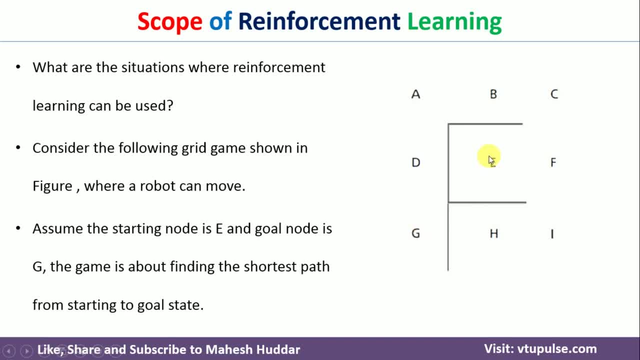 this case, the g is a goal state and is assume that is the place where the agent is present. and if you want to find an optimal path so that the agent can go from this particular state to this one, that's a goal state. in such cases we can use this reinforcement learning. so, uh, whenever 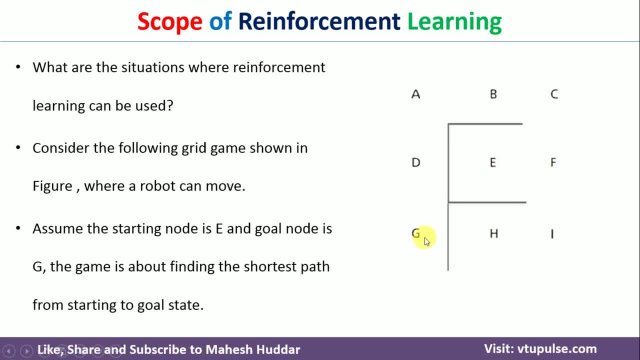 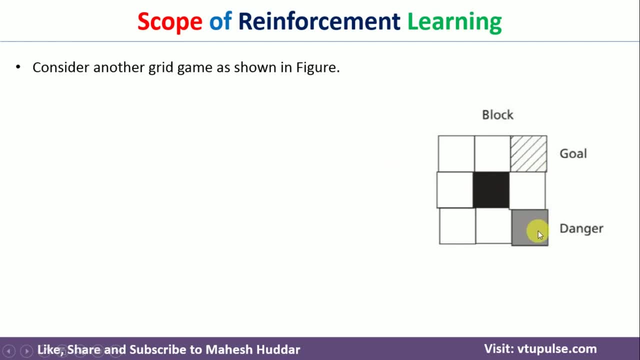 he has to find an action which will lead to this particular goal state here, so that in such cases we can use the other input. let us take one more example. in this case we have been given three kind of things: the- this is the goal state, this is the block, or can say that: 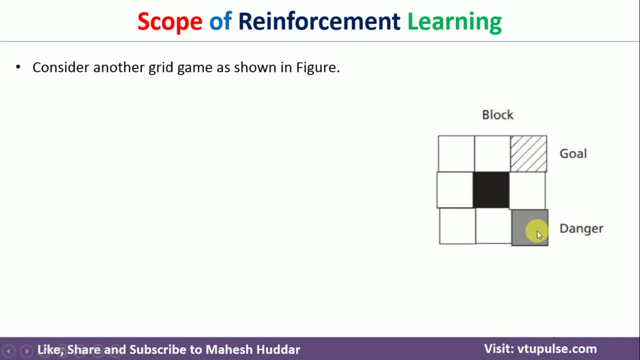 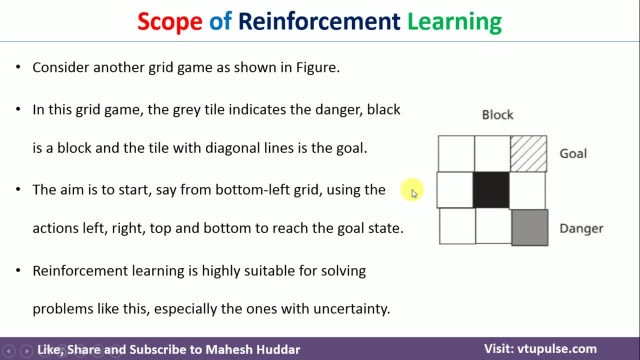 the user cannot cross this particular block here and this is the danger spot here. so, given the agent present in any one of these particular states, we need to find an optimal path so that the user can go through this particular goal over here. so in such kind of the situations we can use. 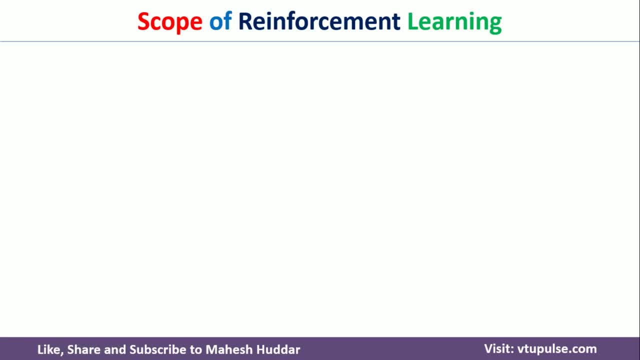 reinforcement learning over here now if you have the data where the complete information is available. for example, you are trying to solve a problem like object detection, face recognition or fraud detection, where a complete information is available in the form of a data set. in such cases, the reinforcement learning is not suitable.